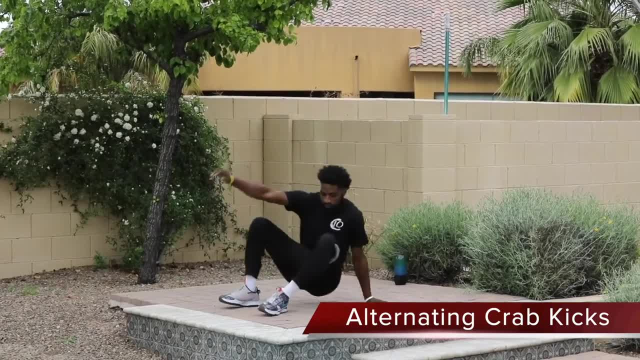 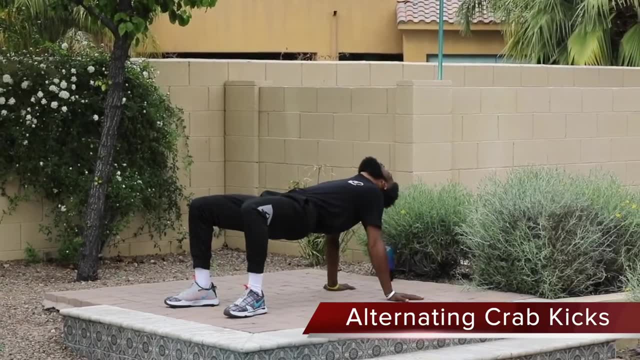 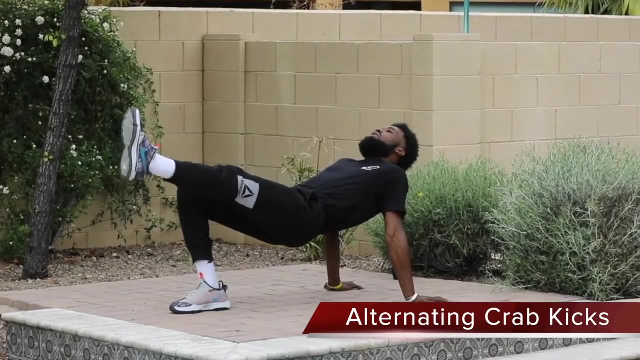 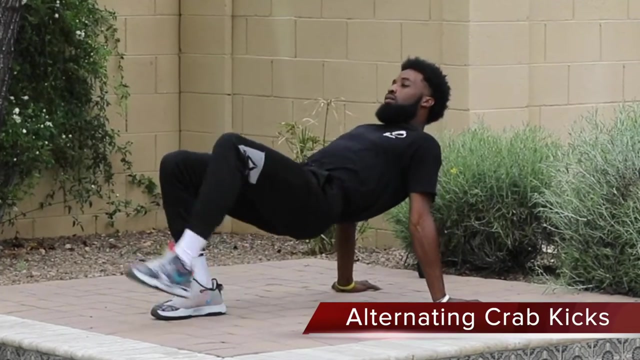 us through alternating crab kicks. Now he will lift his hips up. chin is down like it is. He's going to alternate and kick in right foot, then left foot. He is working his upper body And his hips Chin slightly down. He will continue this for 30 seconds. 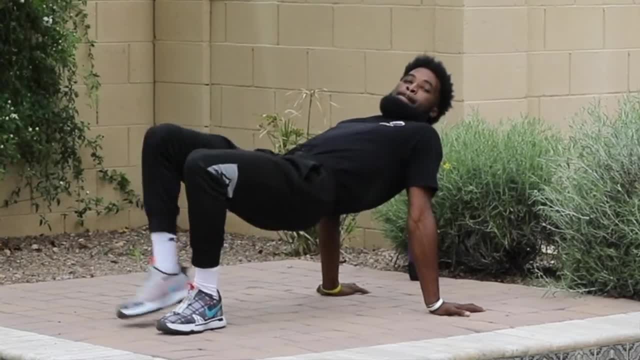 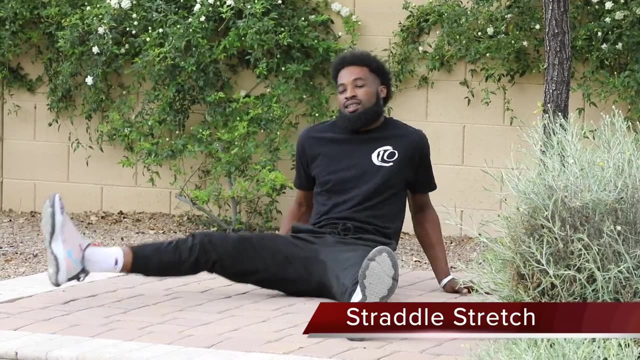 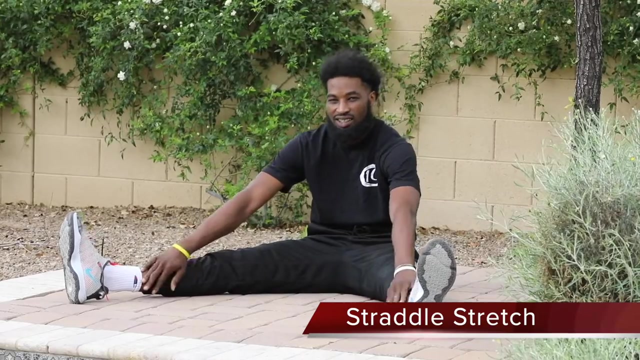 Looking good, Coach K. Coach K is taking us through static flexibility. Our static flexibility today is straddle stretching. You want to make sure that your legs are planted firm on the ground, Your toes are pointed towards your knee And if you would like to challenge yourself, 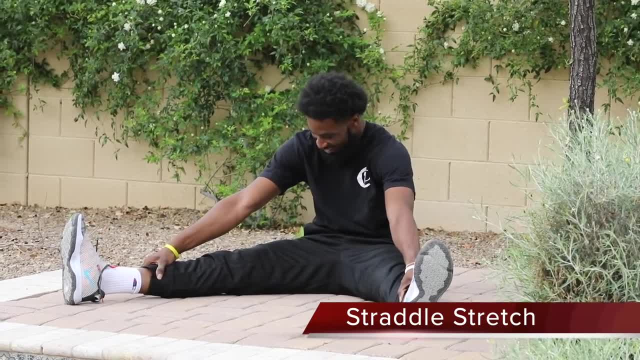 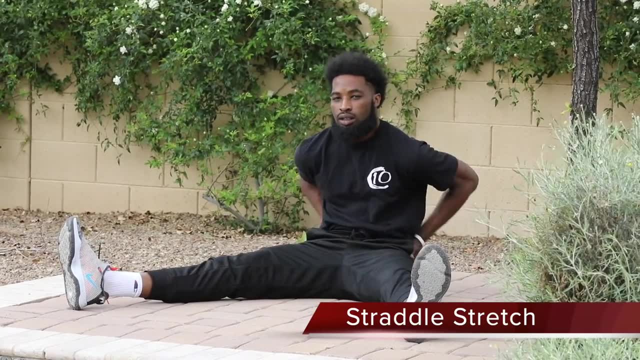 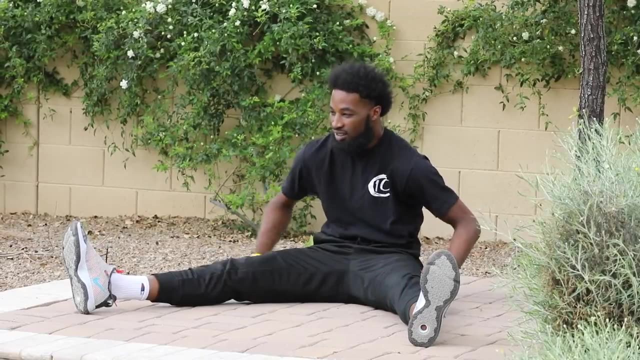 you can touch your toes, or you can touch your shins, or you can touch your knees, or you can just sit up with your back straight and tighten your thighs. You're going to do that for 30 seconds. This stretch is stretching your hamstrings, the muscle that is behind your legs. Coach K is taking. 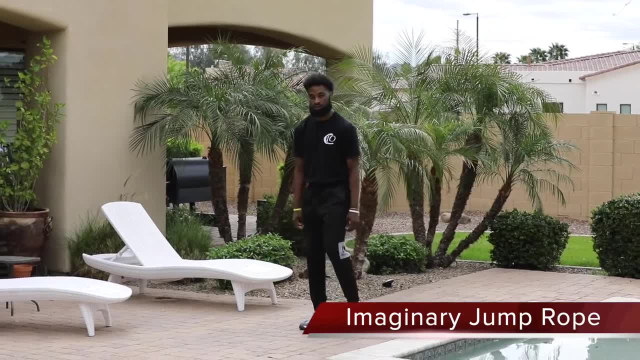 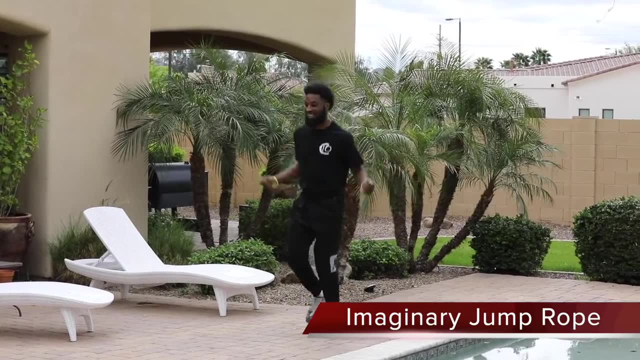 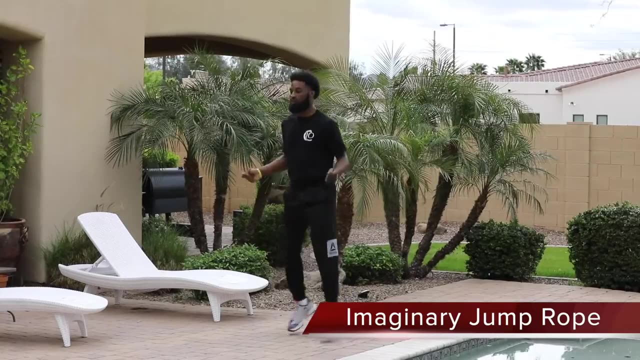 us into imaginary jump rope. Now you have to use your imagination. Take your imaginary jump rope. You can jump rope on one foot. You can walk on your beloved jonhood Four feet, Criss cross, Anything you like. It is your class, it is your day and it is your imaginary jump rope. 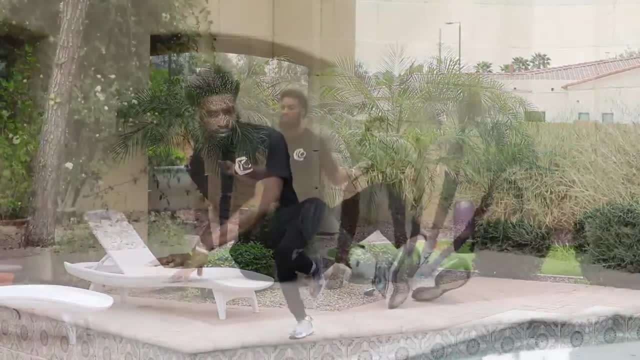 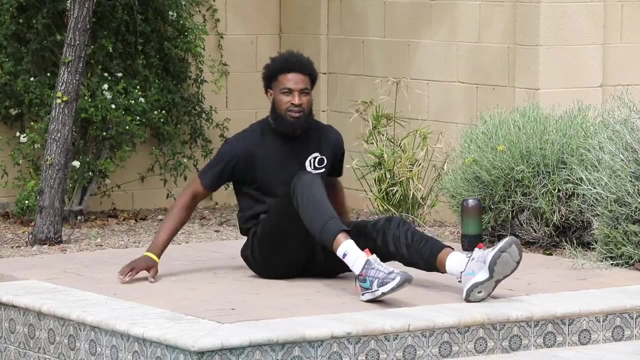 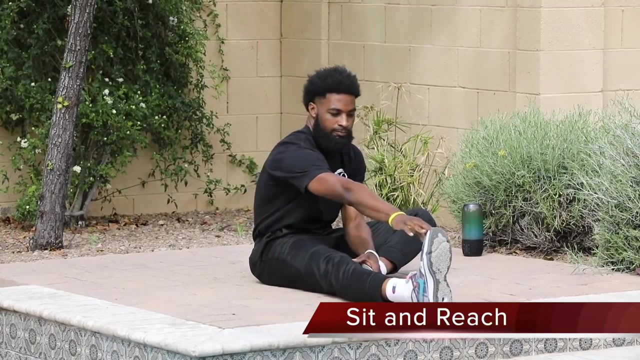 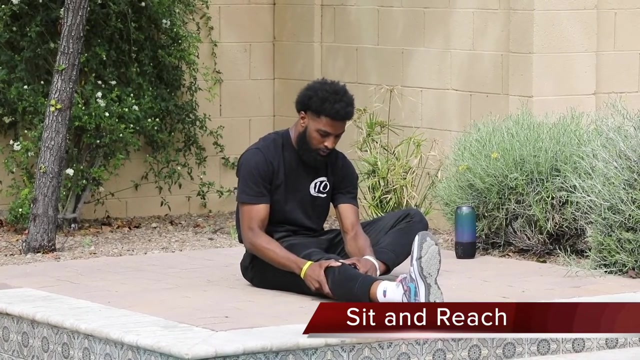 seconds looking good, coach K. coach K is leading us in another static flexibility stretch we are doing: sit and reach. your legs should be in the number four position with your toe pointed towards your knee. you can challenge yourself and touch your toe. you can touch your shin, your knee or you can sit straight with 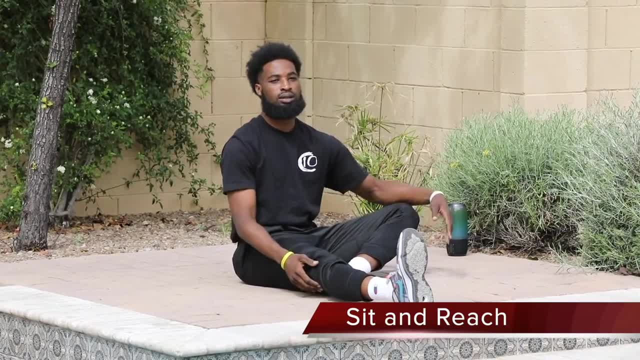 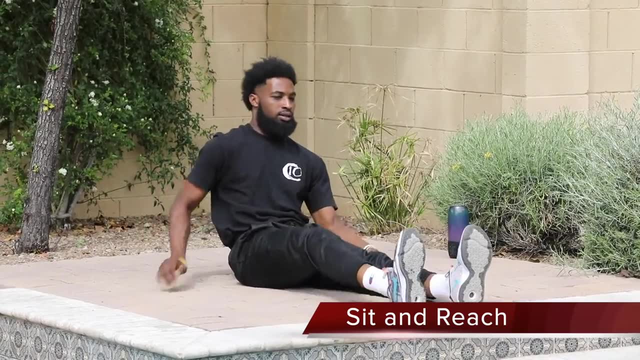 your thigh flexed, if you like. you want to make sure when you stretch that it's a nice, easy stretch and not a pull. you don't want to feel a pull. after a count of 15, you'll switch legs, go to the other leg, same thing, toes, shin. 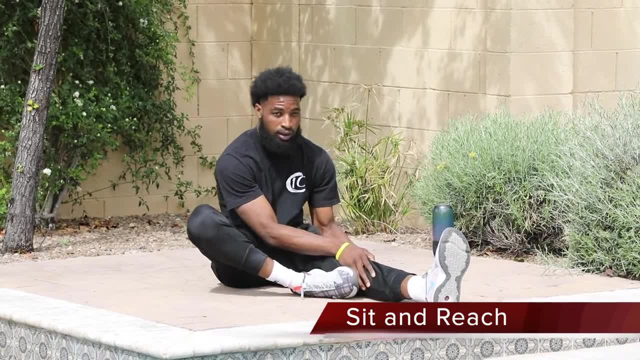 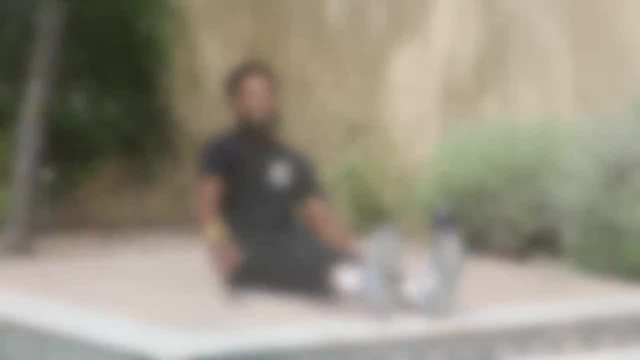 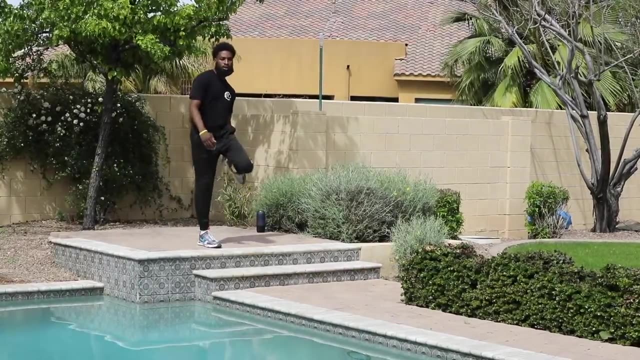 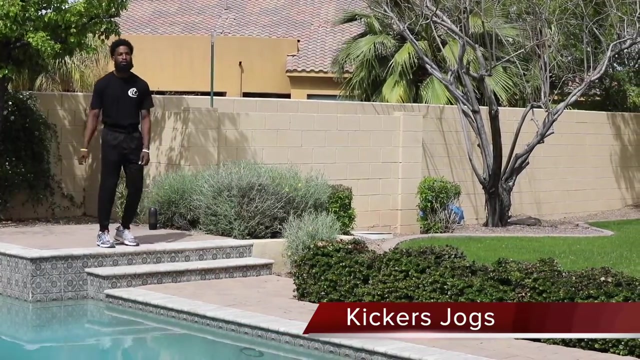 or knee, or straight up with your thigh tightening. thank you, coach K. you looking good. coach K is going to lead us in a static, us into an aerobic activity. This activity is called Kickers Jogs. Now, with Kickers Jogs, it is a light jog, with your foot moving up to your butt. Notice how he's going nice. 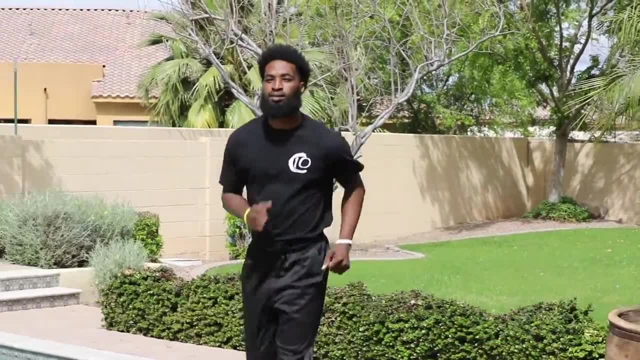 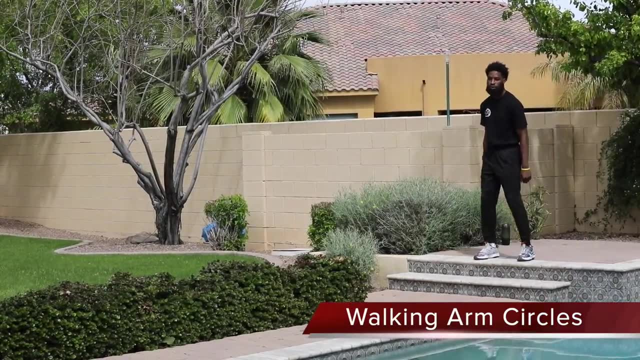 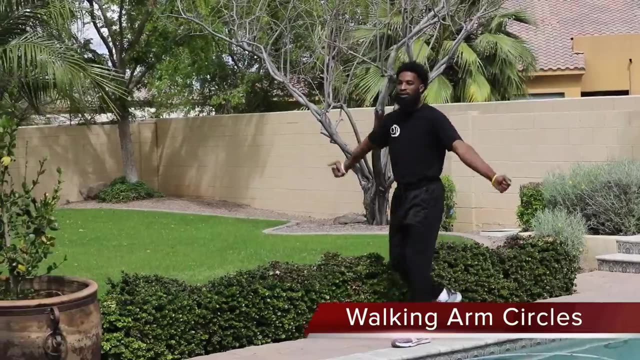 and easy, with his heels coming up nice and high. Do it at a nice, slow, moderate pace. Okay, Coach K, we have another aerobic activity: Walking Arm Circles. Coach K will step down. He will start walking as he turns his arms in a circle motion. Nice and easy, Remember. 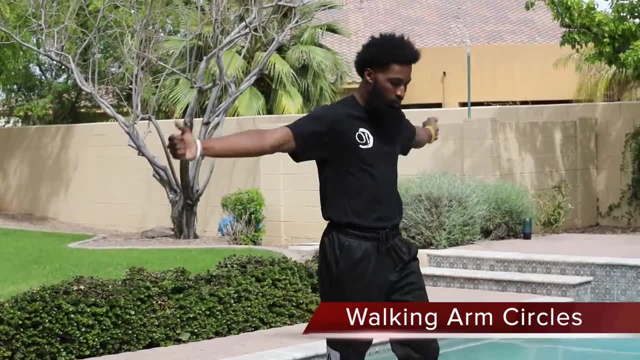 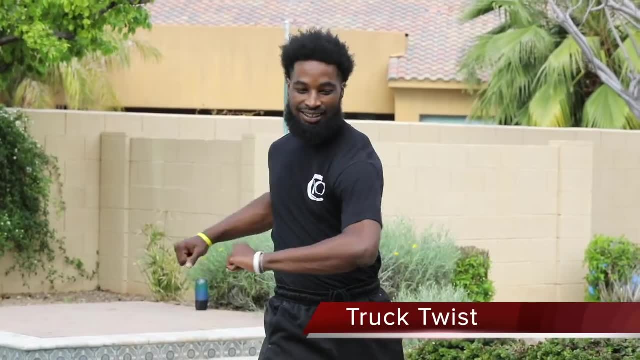 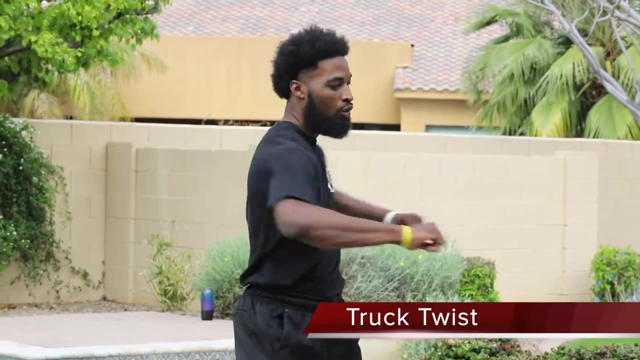 this is a 30-second activity. Okay, Coach K, we are back. We are doing dynamic flexibility right now. We are stretching while in motion. We are doing a trunk twist- Nice and easy- right to left, with your elbows in like an arrow position. 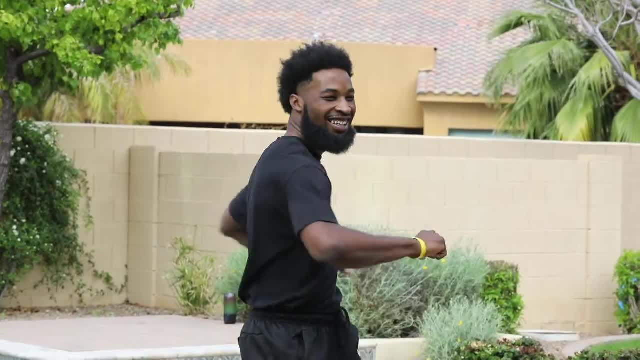 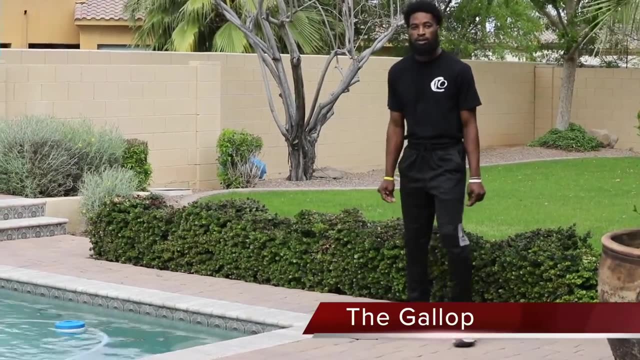 This is an aerobic exercise. This is an aerobic exercise that you should go out and do once a 30-second activity. looking good, coach K, keep it going. okay, now we are galloping, coach K, he will put one foot forward. one foot will always remain in front and you. 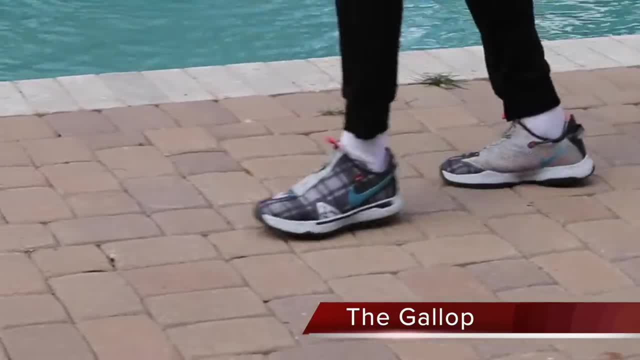 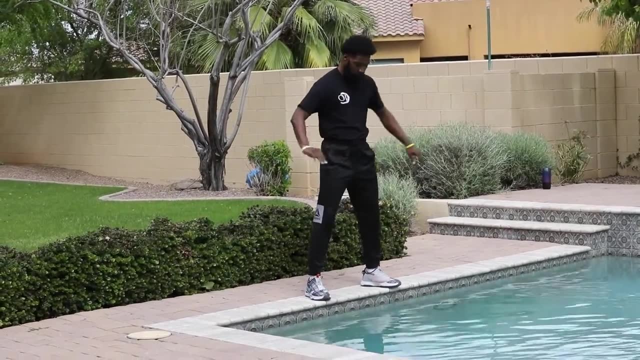 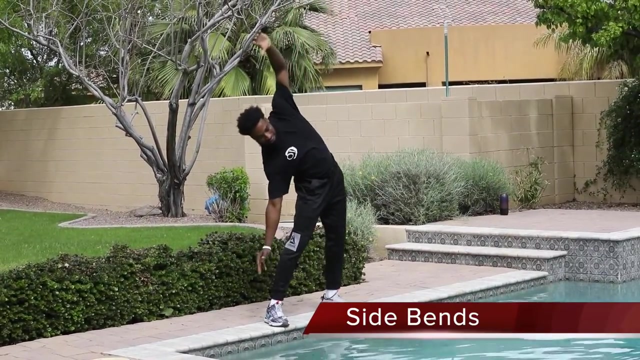 will push off the back foot in a gallop motion. 30 seconds, coach K. we are almost there. we are doing a dynamic flexibility side bends. you can have your arms out like a airplane if you like, and you're going to go down with your hands going. 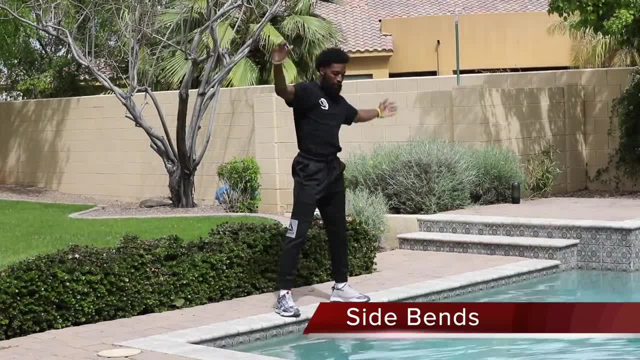 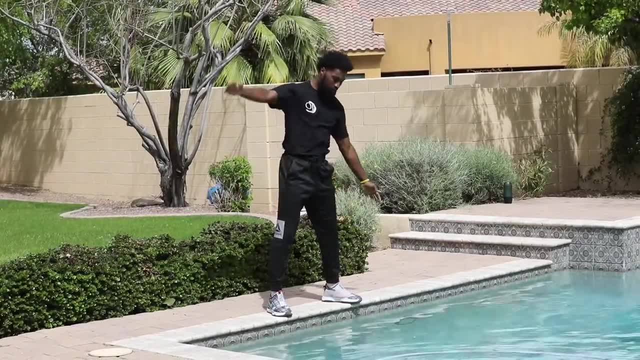 past your knee, stretching your obliques 30 seconds. we're almost there. good job everyone. coach K, we are almost to the finish line. we are going to start. coach K, we are almost to the finish line. we are going to start. we are going to start. 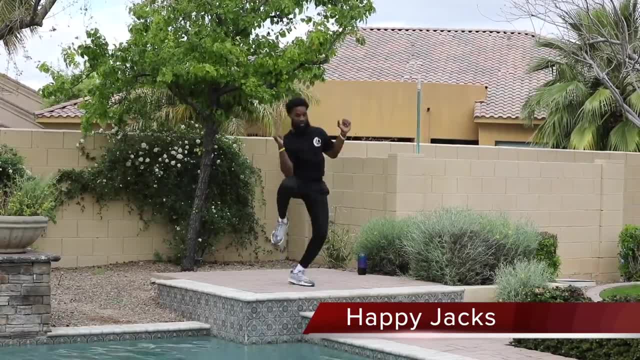 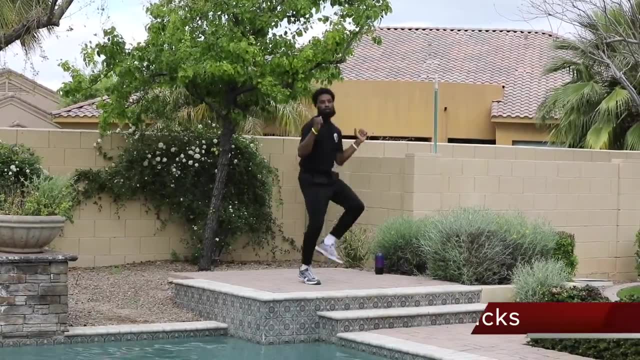 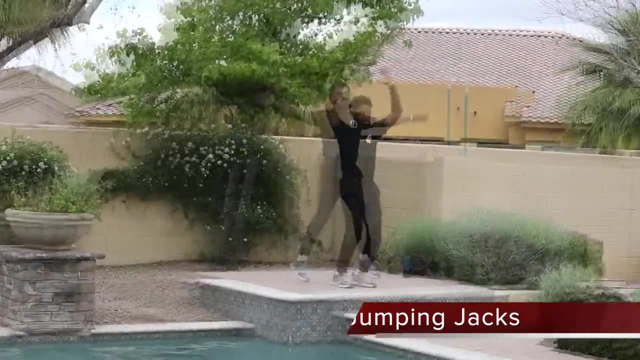 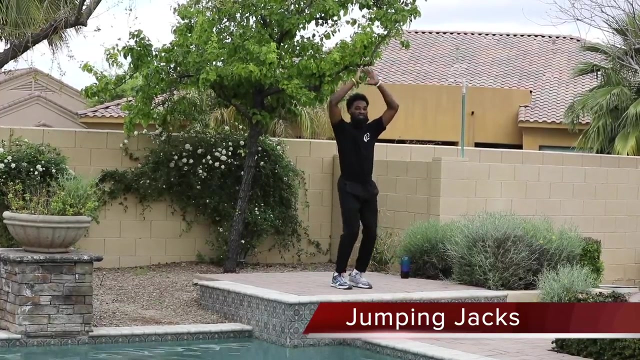 with some happy jacks. make sure those elbows touch those knees, then we can slide into jumping jacks. jumping jacks looking nice, perfectly done. start pencils looking good. coach K, I believe in you. I knew you could do it. great job, perfectly done. okay, here we go, we are. 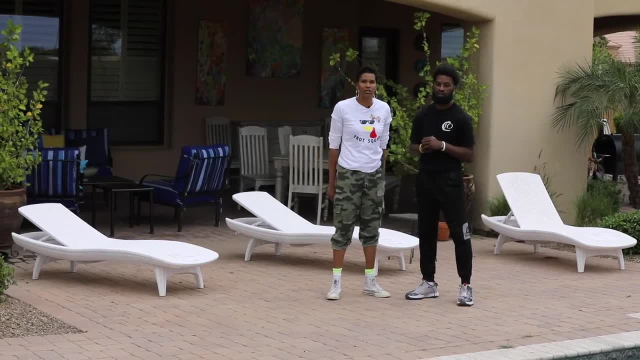 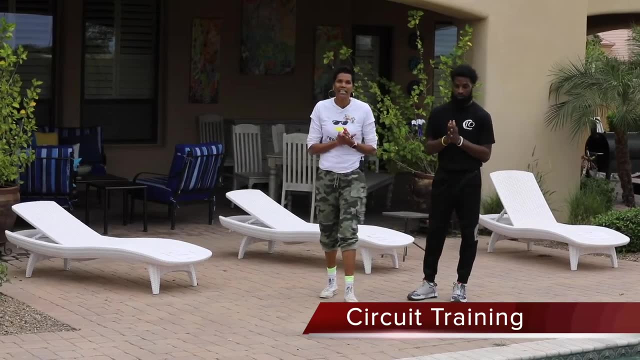 great job, perfectly done. okay, here we go, we are back. we are going to do a circuit back. we are going to do a circuit training course for you today. me miss training course for you today. me miss coach Davis and coach K now. circuit, coach Davis and coach K now. circuit training is one set of a prescribed 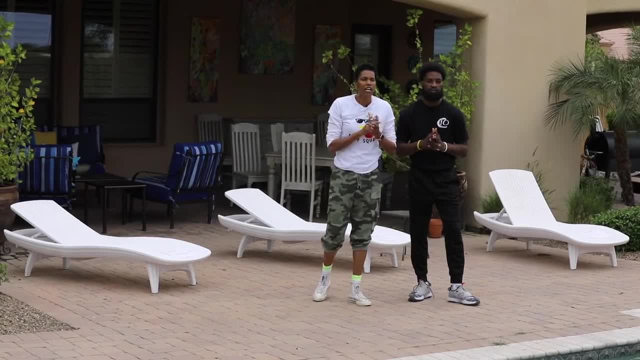 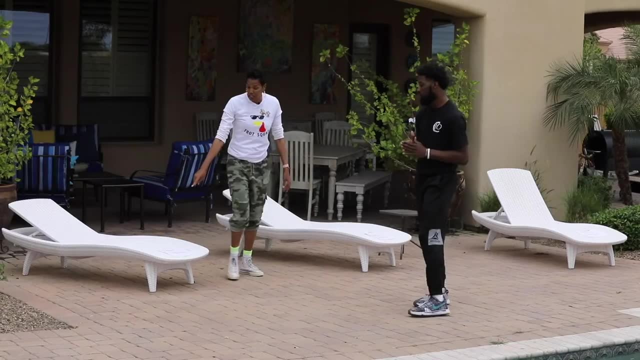 training is one set of a prescribed activity like one circle of motion. okay, activity like one circle of motion. okay, you can have as many activities in it as you can have as many activities in it as you would like. now our first station is: you would like. now, our first station is upper body. second station: lower body, our third. 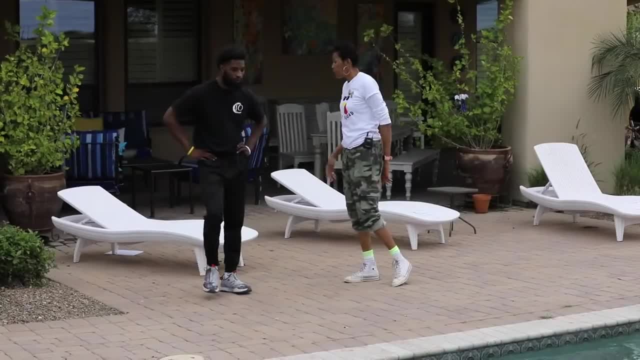 upper body. second station: lower body. our third station is total body station. is total body training. okay, first up in our upper body station. we training. okay, first up in our upper body station. we are going to do the pretzel, are going to do the pretzel stretch. now, when you do your pretzel stretch, you 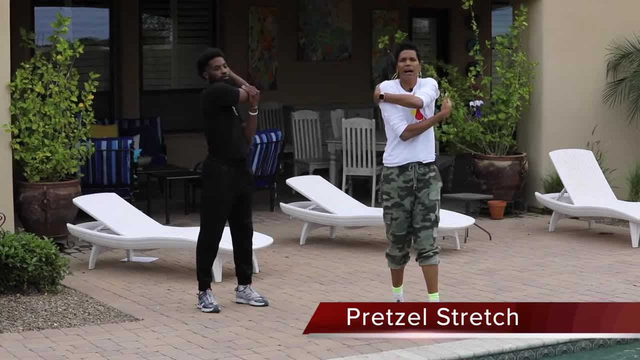 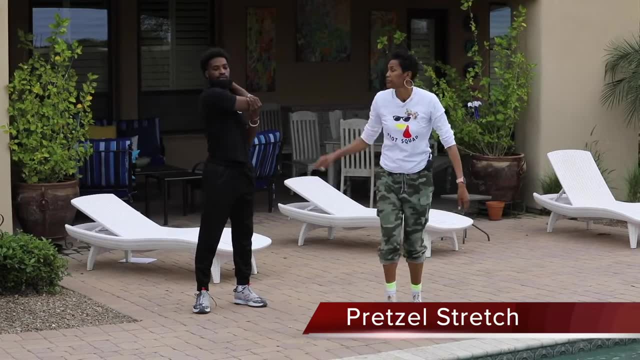 stretch. now, when you do your pretzel stretch, you want to make sure you're on, want to make sure you're on. you're hugging your body and you're taking your. you're hugging your body and you're taking your hand and gently applying hand and gently applying pressure to get the stretch in your deltoids right. 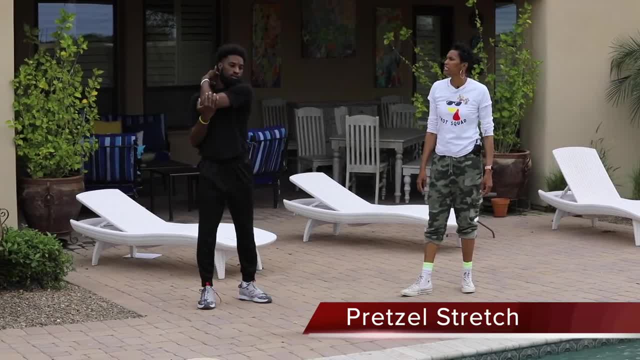 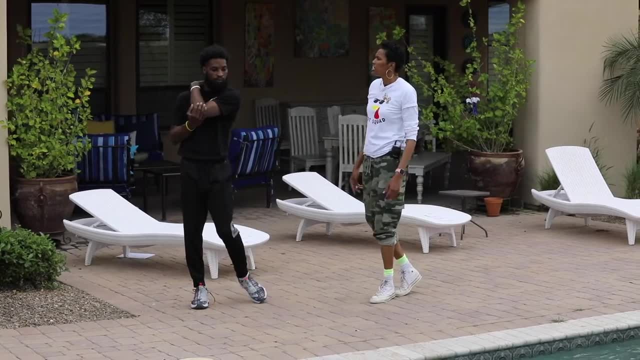 pressure to get the stretch in your deltoids right there. you're going to hold each one there. you're going to hold each one of them for 15, for 15 to count of 15 or so of them, for 15 for 15 to count of 15 or so. okay, next up, we're going to do the 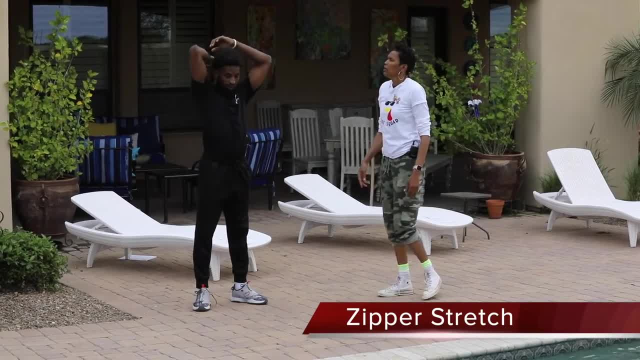 okay, next up, we're going to do the. okay, next up, we're going to do the. zipper stretch our hand will be his hand. zipper stretch, our hand will be his hand. zipper stretch, our hand will be his hand. will be on his elbow, turn around his. will be on his elbow, turn around his. 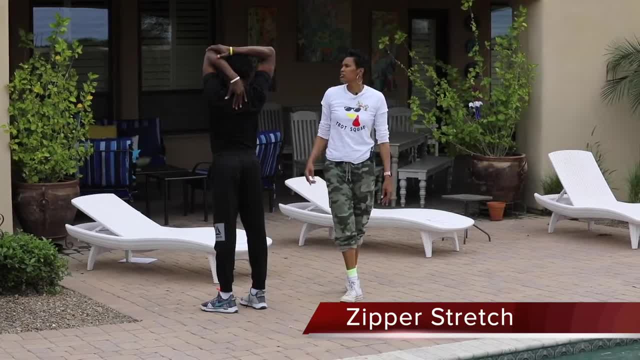 will be on his elbow. turn around: his hand is flat against his back and he is hand is flat against his back and he is hand is flat against his back and he is stretching his triceps and his deltoids- stretching his triceps and his deltoids. 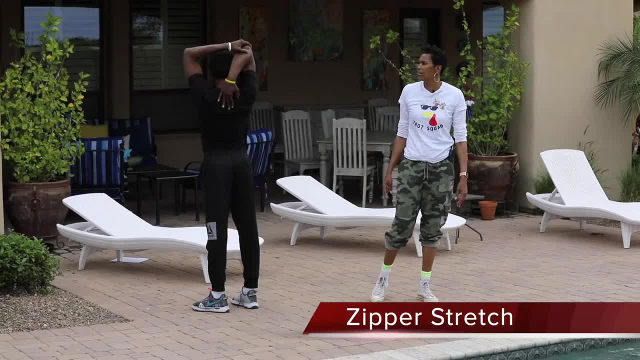 stretching his triceps and his deltoids. you can hold that for 15, then you can. you can hold that for 15, then you can. you can hold that for 15, then you can switch to the other side next stretch. switch to the other side next stretch. 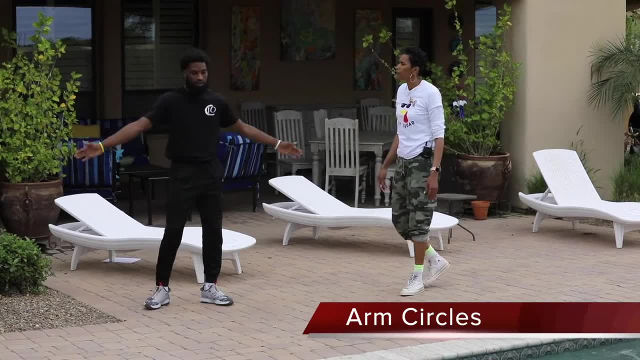 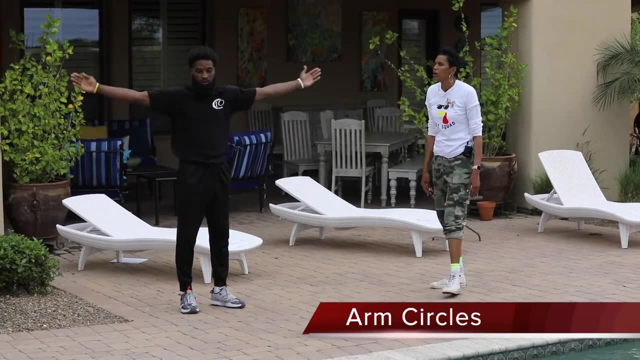 switch to the other side, next stretch. we're doing arm circles. you can do. we're doing arm circles. you can do. we're doing arm circles. you can do. little baby arm circles, our medium arm. little baby arm circles, our medium arm. little baby arm circles, our medium arm circles. but make sure you maintain. 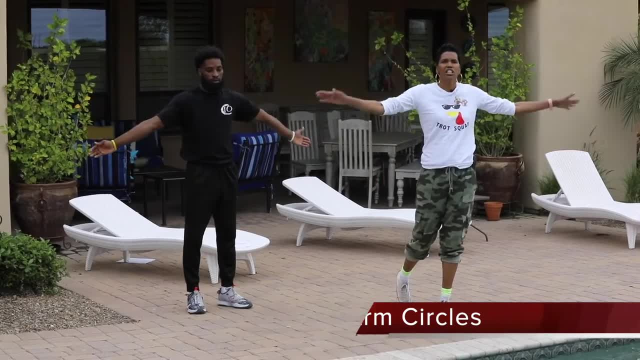 circles, but make sure you maintain circles, but make sure you maintain control. you don't want to do this fast control. you don't want to do this fast control. you don't want to do this fast. it's nice, slow and easy, first up is our. it's nice, slow and easy, first up is our. 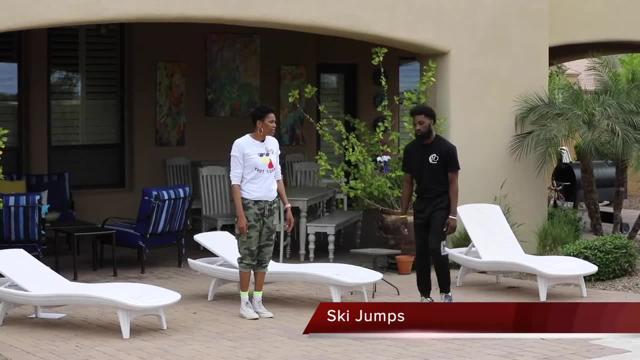 it's nice, slow and easy. first up is our ski jumps. we're going to make sure your ski jumps. we're going to make sure your ski jumps. we're going to make sure your feet are together and you're going to. feet are together and you're going to. 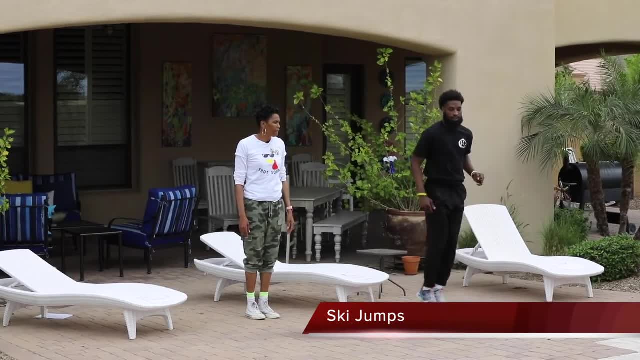 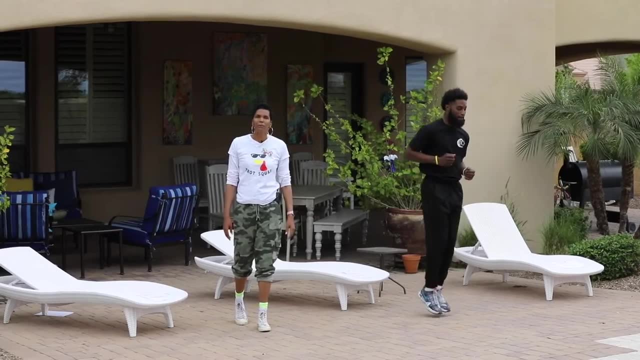 feet are together and you're going to jump slightly side to side. nice and rhythm rhythmically next up. nice and rhythm rhythmically next up. nice and rhythm rhythmically next up. we are going to do, we are going to do, we are going to do rocking, rocking. 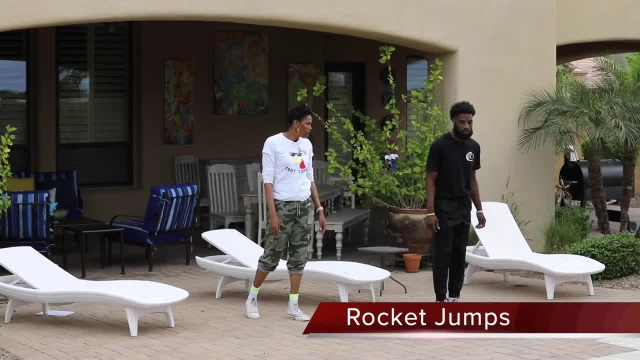 rocking jumps, rocket jumps. your feet should be jumps, rocket jumps. your feet should be jumps, rocket jumps. your feet should be shoulder width apart, shoulder width apart, shoulder width apart. you're going to touch the ground with. you're going to touch the ground with. you're going to touch the ground with your hands flat. 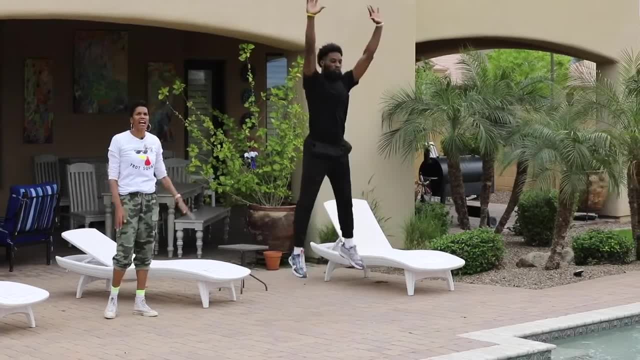 your hands flat, your hands flat. bend down, bend your knees, and then you're bend down. bend your knees, and then you're bend down. bend your knees and then you're going to explode up as high as you can, going to explode up as high as you can. 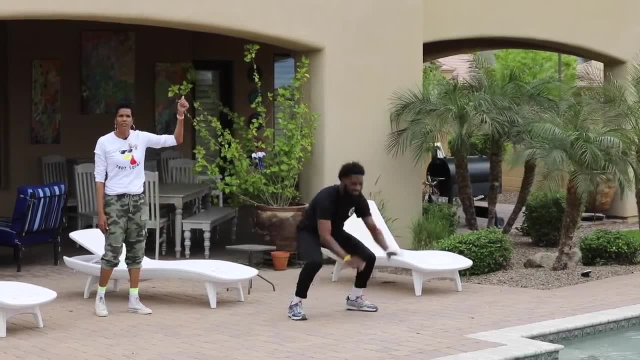 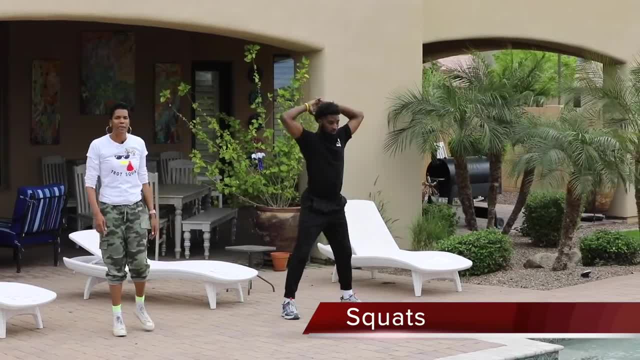 elbows pointed like an arrow. elbows pointed like an arrow. there you go, looking nice, nice and easy. there you go, looking nice, nice and easy. there you go, looking nice, nice and easy, and i know you guys are going to enjoy, and i know you guys are going to enjoy. 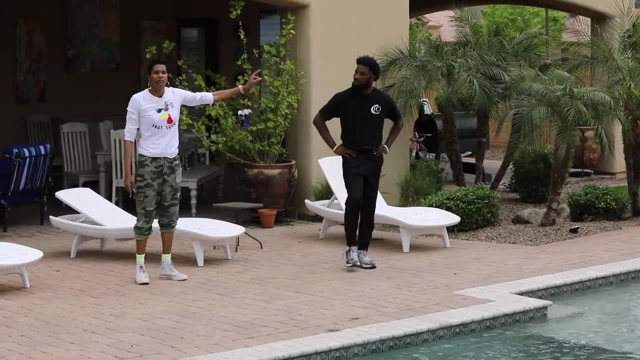 and i know you guys are going to enjoy this, this, this mr marquis is going to give you a. mr marquis is going to give you a. mr marquis is going to give you a refresher course on how to do a burpee. refresher course on how to do a burpee. 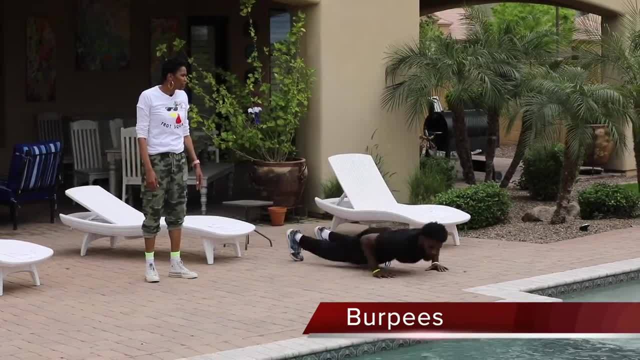 refresher course on how to do a burpee. he's going to jump up, he's going to jump up. he's going to jump up, he's going to kick out, then he's going to, he's going to kick out, then he's going to, he's going to kick out, then he's going to go to a push-up. there you go. 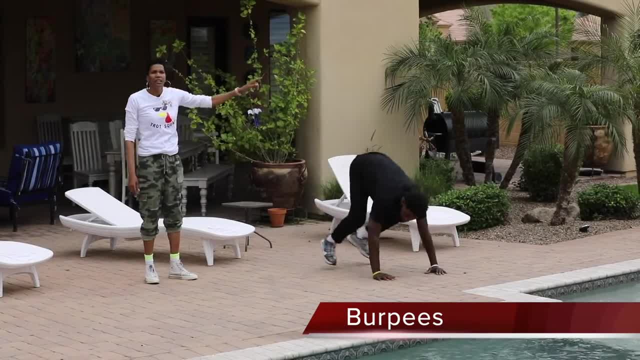 go to a push-up, there you go. go to a push-up, there you go. jump up, kick out, go down to a push-up. jump up, kick out. go down to a push-up. jump up, kick out, go down to a push-up. that's your burpee. here's how you modify. 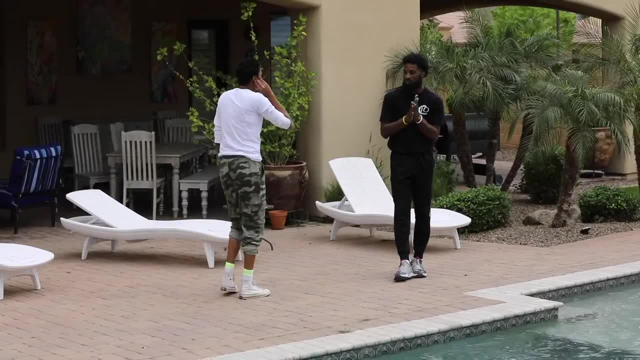 that's your burpee. here's how you modify that's your burpee. here's how you modify that. if that's a little too much for you, that, if that's a little too much for you, that, if that's a little too much for you, you're gonna go jump up. 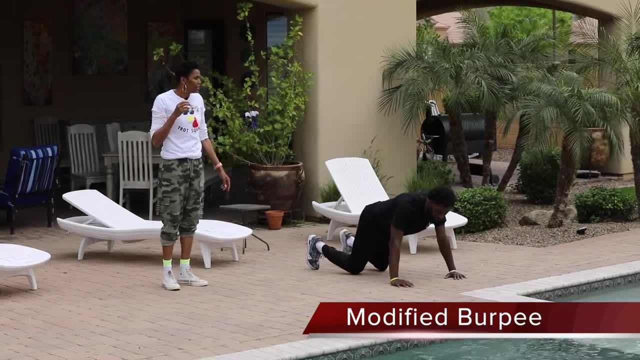 you're gonna go jump up. you're gonna go jump up, kick out, kick out, kick out, and then you're gonna go to your knees and then you're gonna go to your knees, and then you're gonna go to your knees, do your push-up, do your push-up. 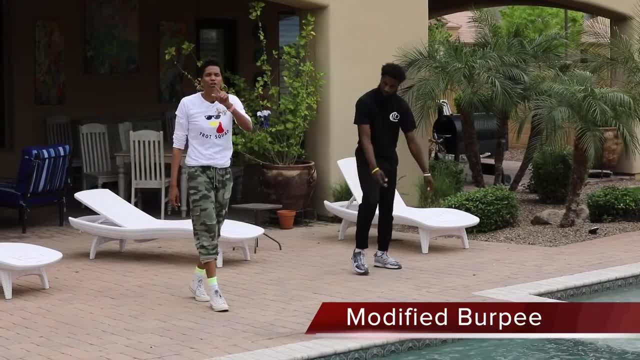 do your push-up there, you go, there, you go there, you go like that, and i know you can do it next like that, and i know you can do it next like that and i know you can do it next up. we are going to do mountain climbers. 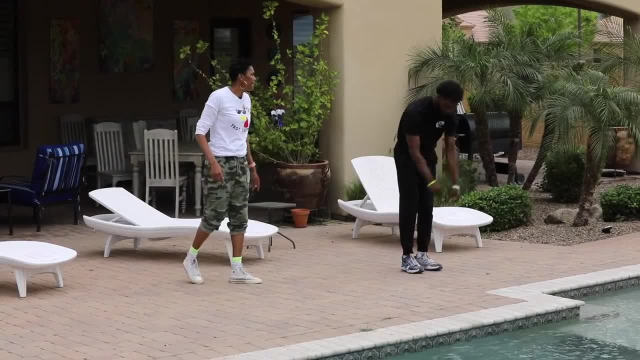 up we are going to do mountain climbers. up we are going to do mountain climbers- everybody's favorite. so everybody's favorite, so everybody's favorite. so, mr marquis coach kate will get in the. mr marquis coach kate will get in the. mr marquis coach kate will get in the push-up position and he's going to run. 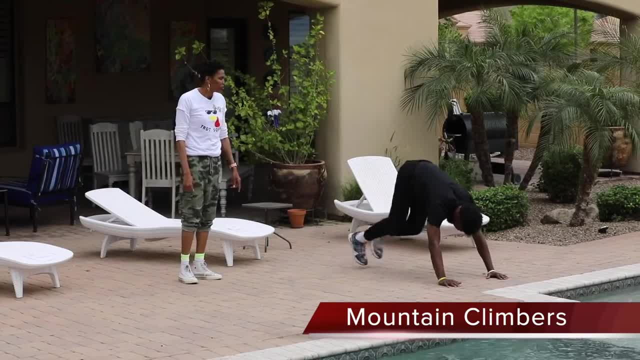 push-up position and he's going to run push-up position and he's going to run in place, in place, in place. nice and smooth, nice and smooth. i like nice and smooth, nice and smooth. i like nice and smooth, nice and smooth. i like that. i like that you can do that. that i like that you can do that. that i like that you can do that anywhere. you can do it outside, you can anywhere. you can do it outside. you can anywhere you can do it outside. you can do it in the living room, you can do it. do it in the living room, you can do it. 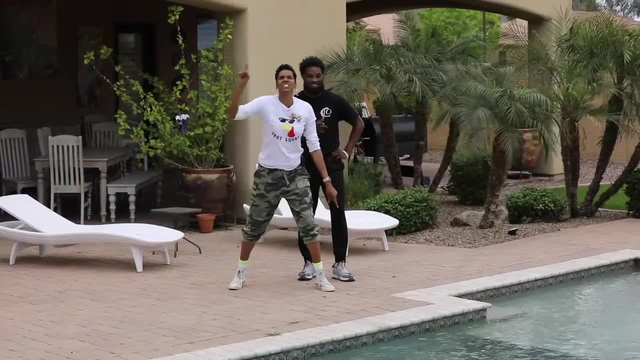 do it in the living room, you can do it in the hallway. you can do the last in the hallway. you can do the last in the hallway. you can do the last activity of activity, of activity of today: our jumping jacks. you already know today, our jumping jacks, you already know. 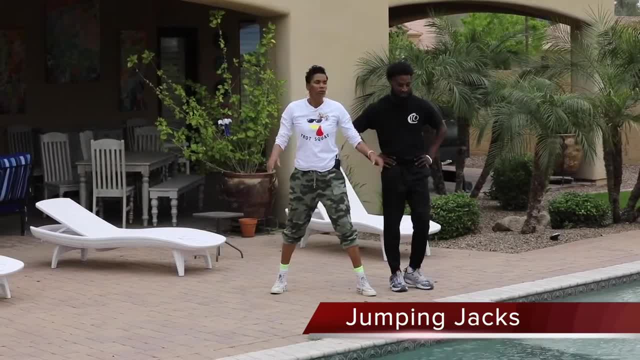 today our jumping jacks. you already know how to do it, because we did it in warm. how to do it because we did it in warm. how to do it, because we did it in warm, up, so, up, so up. so, mr marquis, take it away, coach k. 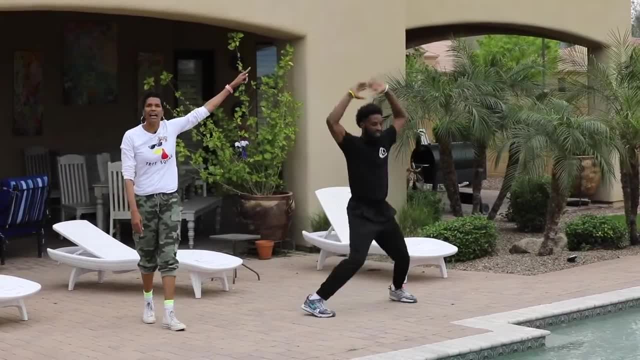 mr marquis, take it away, coach k. mr marquis, take it away, coach k. let's do this, let's do this, let's do this. look how his hands are going up nice. look how his hands are going up nice. look how his hands are going up nice and high over his head, touching coming. 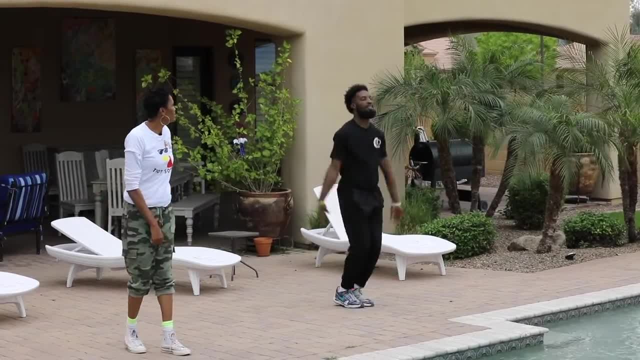 and high over his head, touching, coming and high over his head, touching, coming back with his hands to his side, back, with his hands to his side, back, with his hands to his side. looking nice, looking nice, looking nice. thank you, coach k, thank you, coach k, thank you, coach k. now each one of these stations. 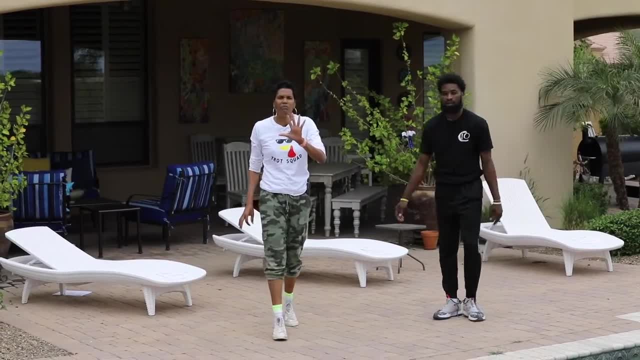 now each one of these stations, now each one of these stations. you will stay there for five minutes. you will stay there for five minutes. you will stay there for five minutes. you stay there for five minutes. you can you stay there for five minutes. you can you stay there for five minutes. you can do all three activities one at a time. 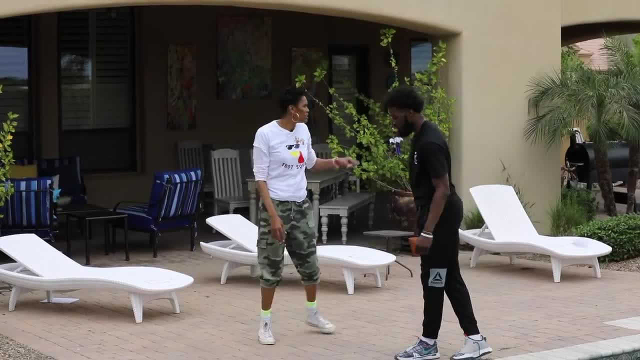 do all three activities one at a time. do all three activities one at a time, five minutes each. or you can do one five minutes each, or you can do one five minutes each, or you can do one activity five minutes. move to the next activity. five minutes. move to the next. 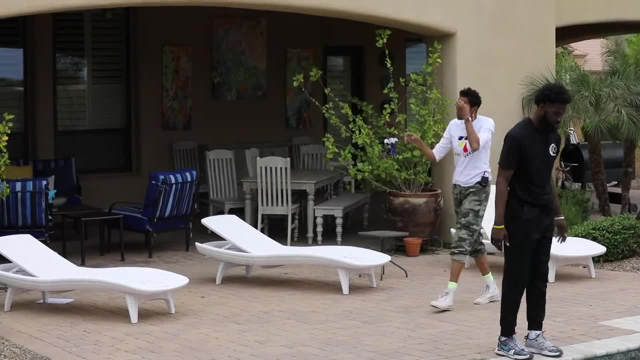 activity five minutes. move to the next activity five minutes. next activity: five activity, five minutes. next activity: five activity, five minutes. next activity: five minutes, minutes, minutes. or you could do one station on monday, or you could do one station on monday, or you could do one station on monday, one station on tuesday, one station on 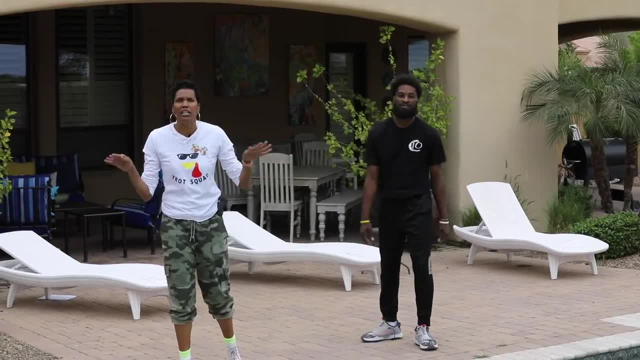 one station on tuesday. one station on one station on tuesday. one station on wednesday: wednesday, wednesday. it's however you want to do it and it's it's however you want to do it and it's it's however you want to do it and it's your.